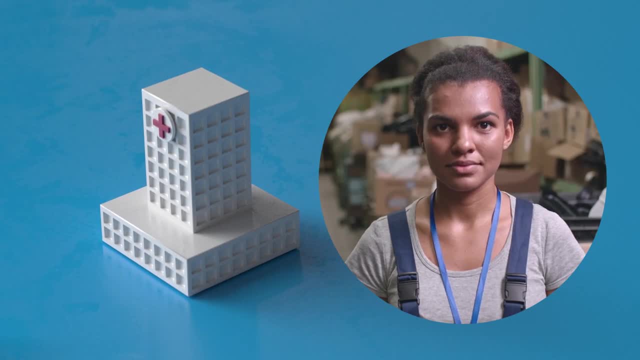 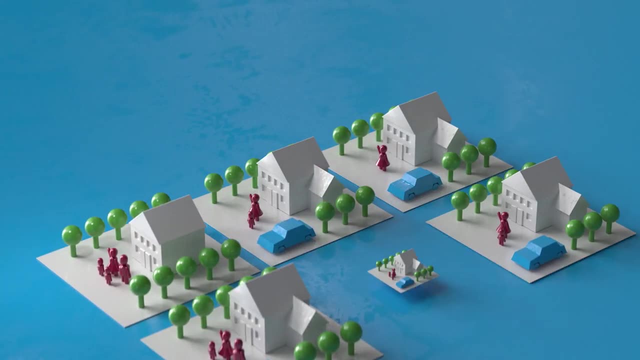 free people from the need to have many children to support them, And access to modern products and contraception means that they can choose to have fewer. In rich countries, where our impact is so excessively high, we can make a critical difference by having smaller families. 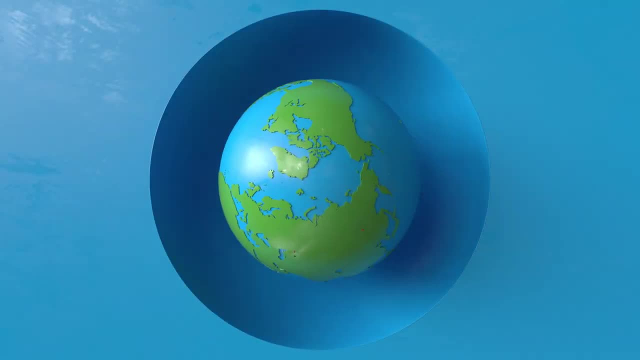 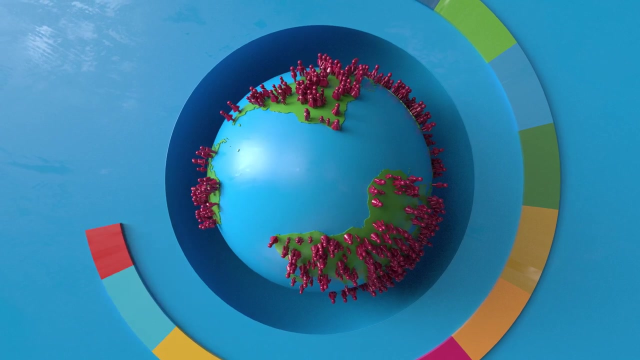 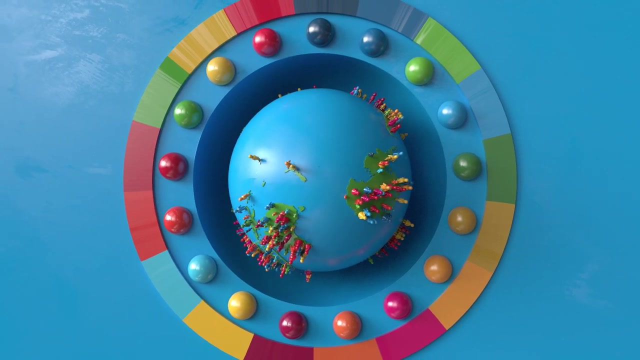 alongside reducing our runaway consumption. Achieving a sustainable global population matters. If we do, we can all have the dignity, security and well-being envisioned by the Sustainable Development Goals. We must not fail. Let's invest in and celebrate it. Let's invest in and celebrate it. 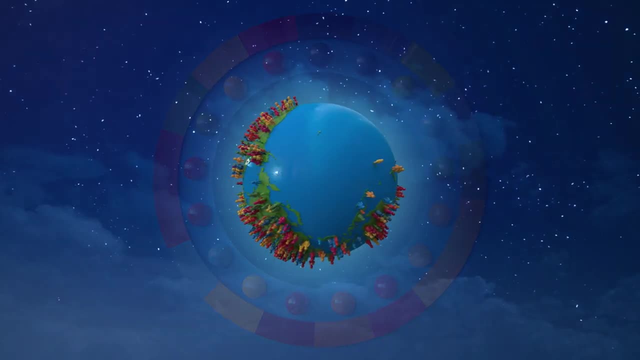 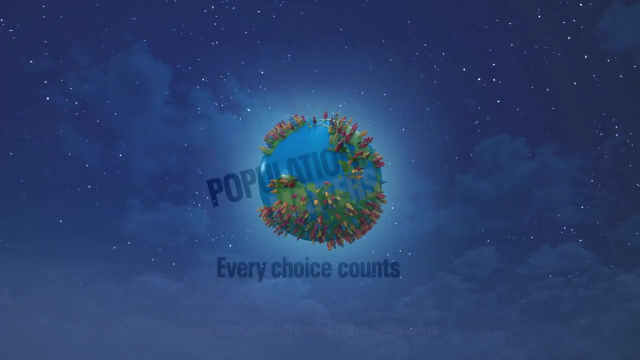 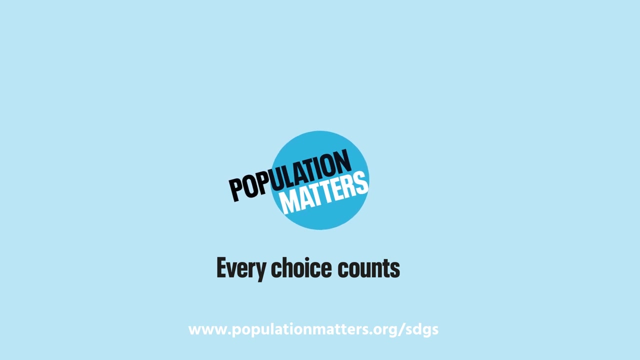 Let's celebrate solutions that empower people to choose smaller families, make their lives better and protect our only home Today, tomorrow and forever. Visit populationmattersorg slash stgs to find out what you can do. 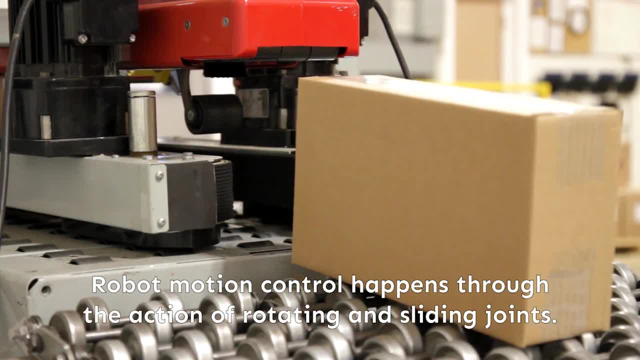 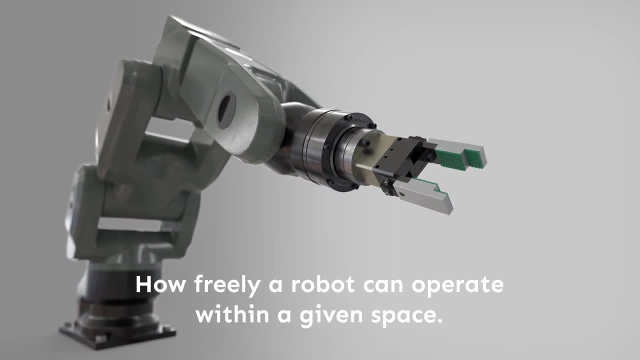 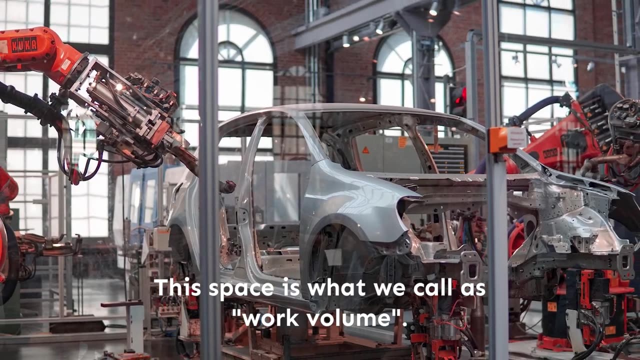 Robot's motion control happens through the action of rotating and sliding joints. The relative motion of all the joints in a robot decides how freely a robot can operate within a given space. This space is what we call as work volume. Work volume protects the robot. 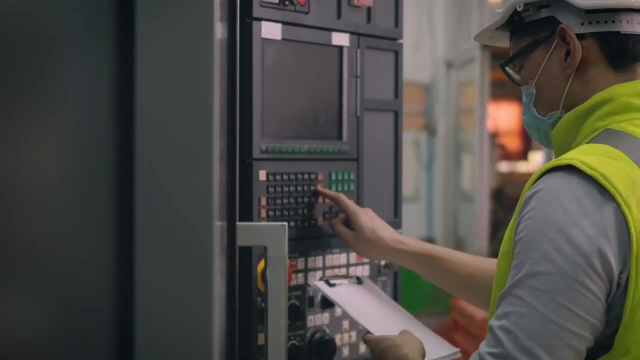 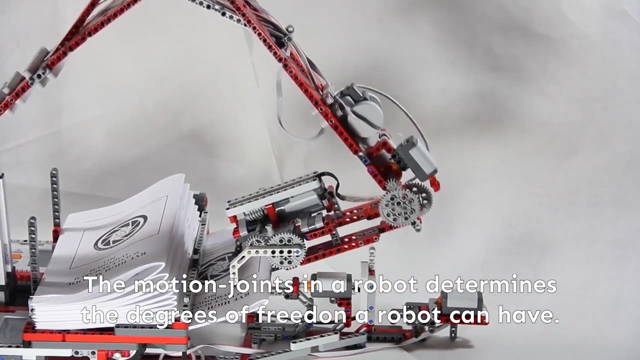 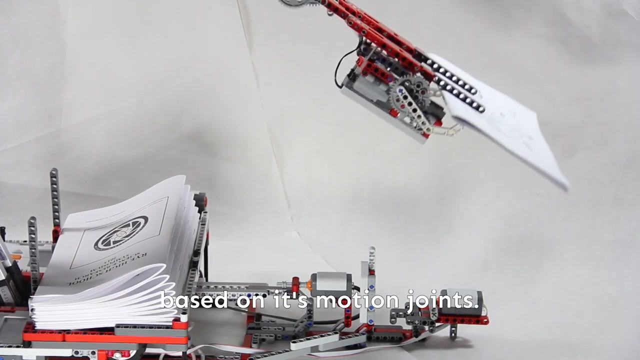 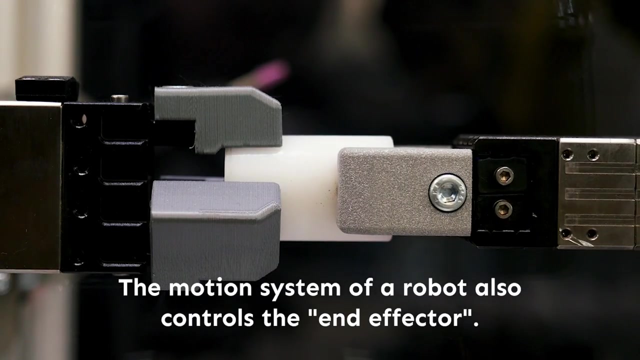 as well as the person working with the robot. The motion joints in a robot determine the degrees of freedom a robot can have. Degrees of freedom means number of individual movements a robot contains based on its motion joints. It could be either linear or rotational motion. The motion system of a robot also controls 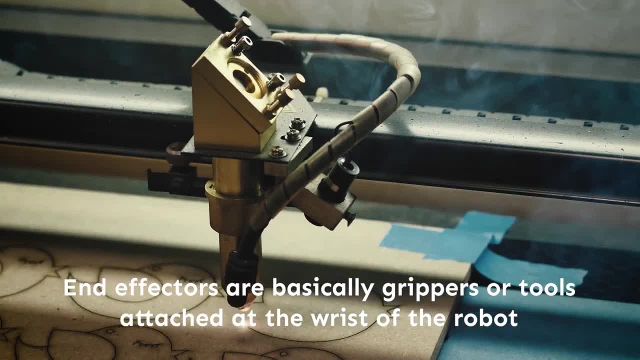 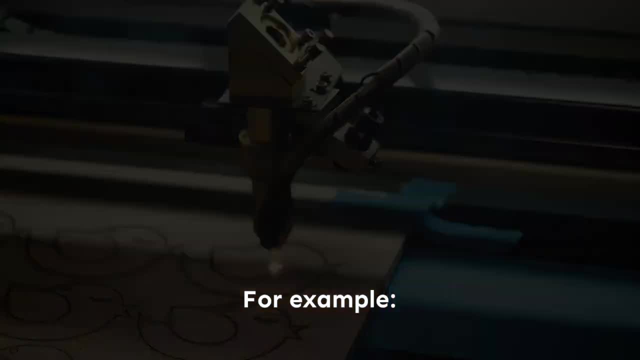 the end effector. End effectors are basically grippers or tools attached at the wrist of the robot. The end effectors are basically grippers or tools attached at the wrist of the robot robot and used for some job. For example, we can take a robot that polishes glass using a grinding. 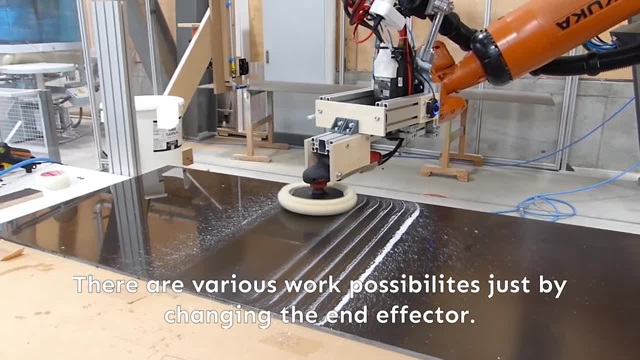 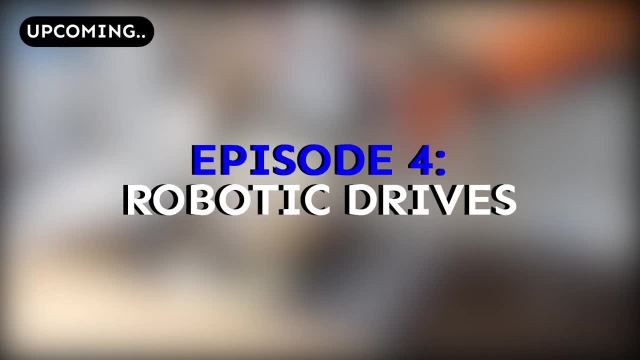 machine as its end effector. There are various work possibilities just by changing the end effector.